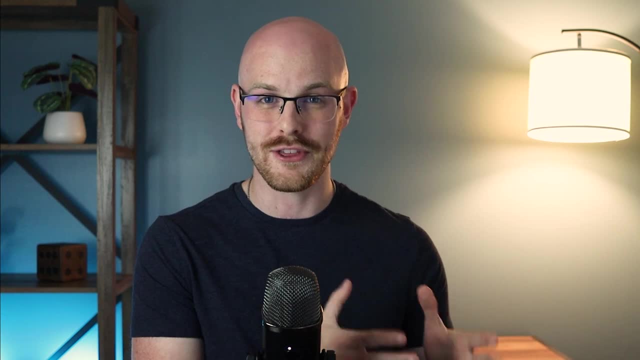 So an API is kind of like a middleman. Let's say you have you over here, you're the user and you want data from this company And they have this API set up And in this API they're going to show you exactly what you are allowed to take and how often you're allowed to. 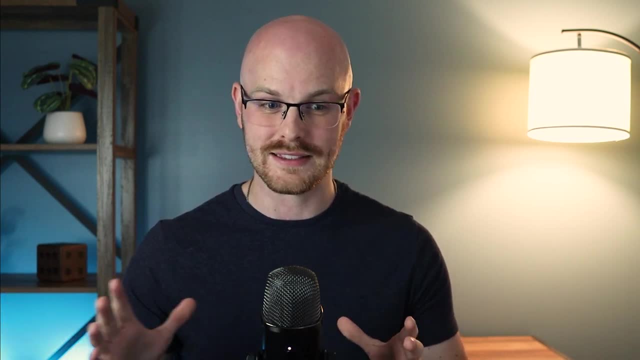 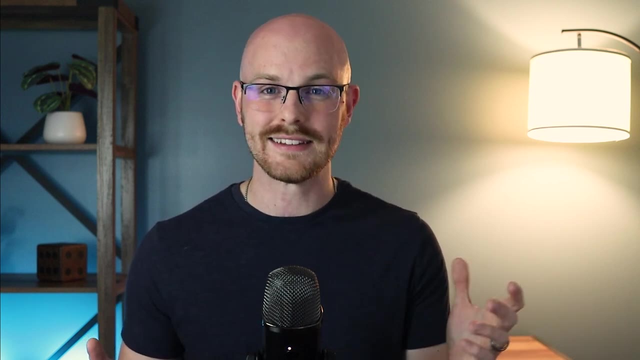 take it And they're not going to show you everything that they have on the client side, because there are things that they don't want you to have access to. So it really keeps both parties happy, because the user can still access the data and use the data, But this company doesn't. 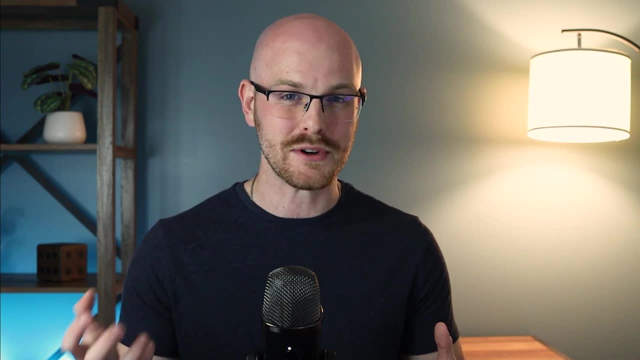 take all the data, So it's going to show you exactly what you are allowed to take and how often, the risk of opening up all their databases and everything. So it's a lot more secure. So, to give you a metaphor for all of this, imagine you're going to a butcher shop. 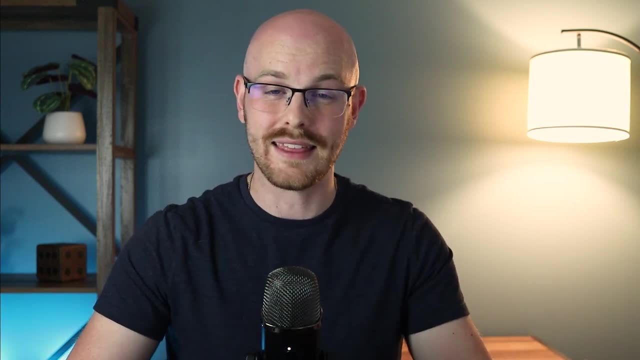 and you know they have all those big display windows of all the different types of meats that they have available And you call the butcher over and you say, Hey, I want this, this and this, And he goes back and he prepares it for you And then he brings it to you and you are a happy customer. 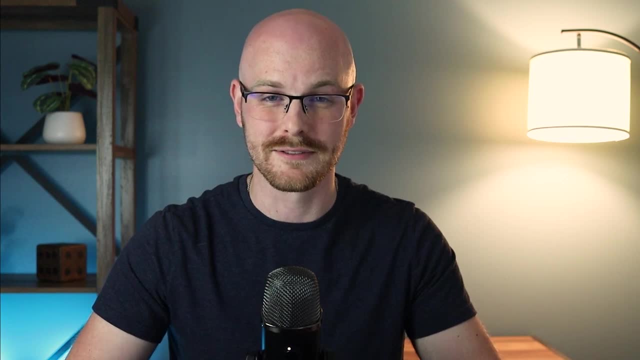 And he is happy because you are buying his products and using his products. And that's basically what an API is. You're not the one going back behind the counter and getting things for yourself and messing everything up. You know that butcher is the one who's going to go get it for you and make sure everything is done. 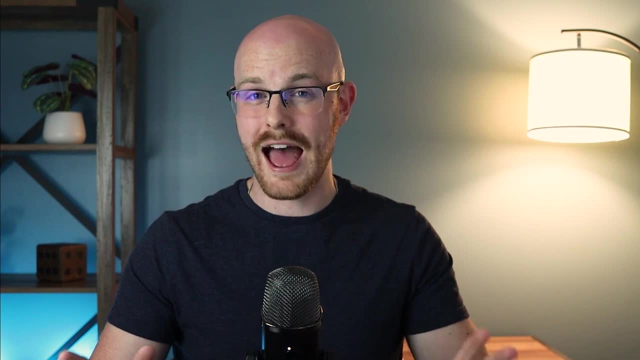 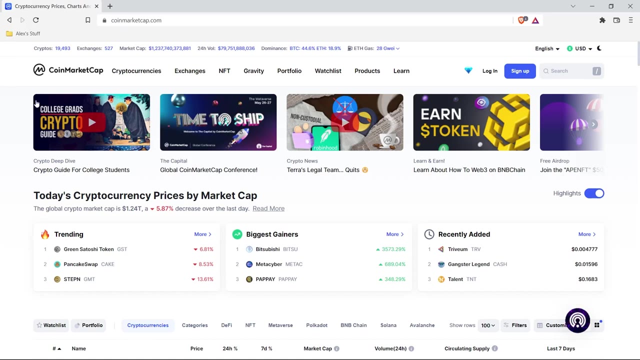 properly. I know that was a fantastic metaphor and you guys all really enjoyed that, but let's jump onto my screen. I'm going to show you how to actually use an API. All right, So to show you how to use an API, we're going to be taking a look at coin market cap And this, basically, is a website. 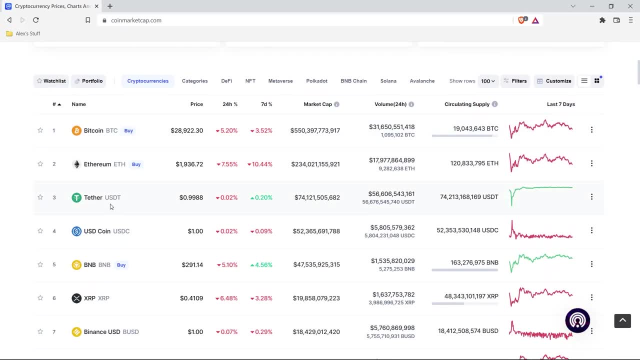 that tracks cryptocurrencies. So over here we have all these different cryptocurrencies and we have their prices, their market caps, volume, circulating supply. Now, if you don't, or if you're not into crypto, you may not know what any of this is. 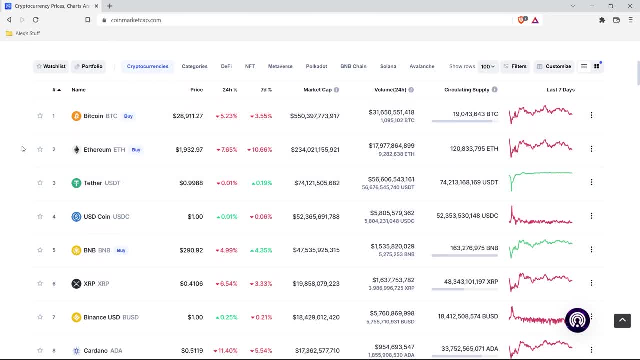 But it's data. You know, here are the columns, here's the data, And we want to use that data. So we want to take that data for, let's say, just a personal project, or we want to put it up on our 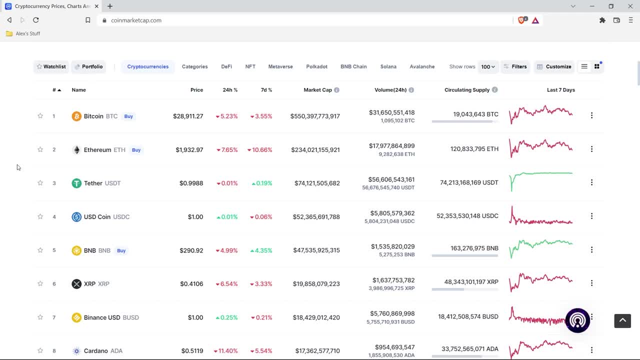 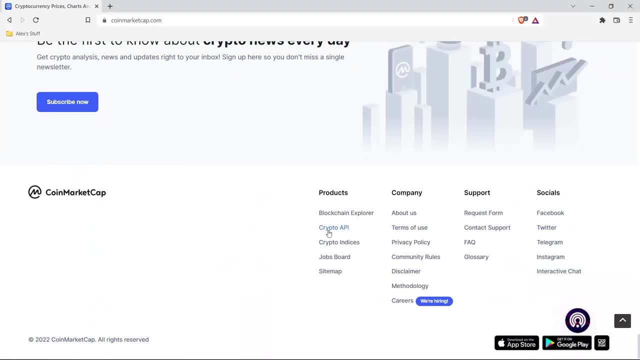 own website and display this. So we want this information, And so what we're going to do is we're going to go all the way down to the bottom. Stick with me, And under products we have this crypto API. So let's go ahead and click on that And it's going to take you to their kind of their. 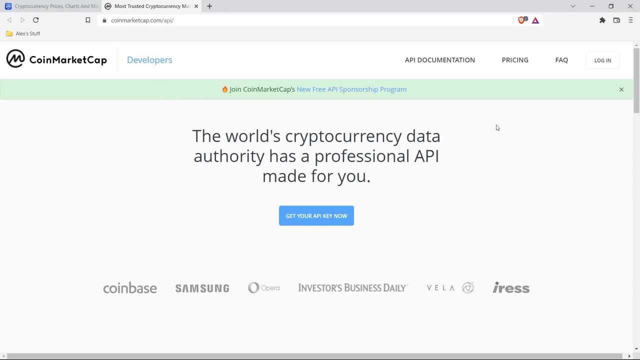 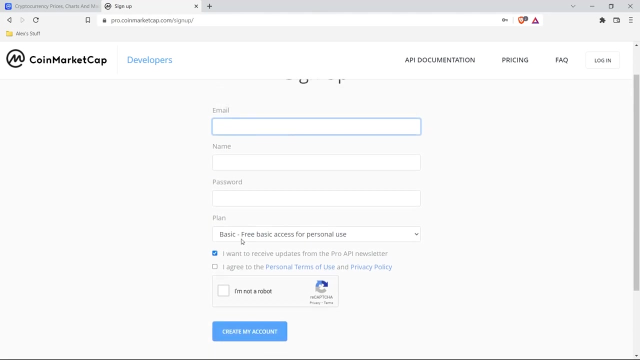 developer section. Now, all you have to do in order to get into the crypto market cap, you're going to have to sign up, So you're going to have to create a free account and that's all you have to do. You can just say: you're a hobbyist and you want this data and you don't want newsletters. 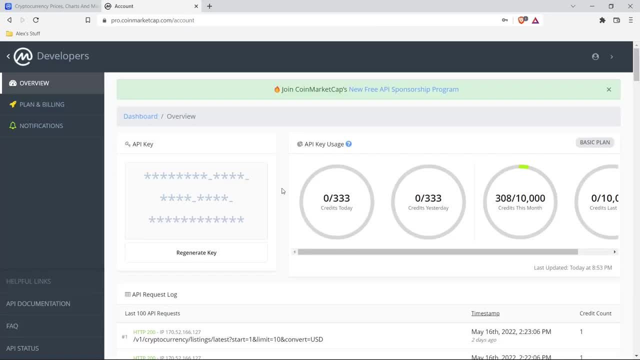 and you're going to create an account. Now I already have an account, so I'm going to log in really quick. So this is our dashboard And right over here we have our API key and you can copy this key or you can generate a new key whenever you want to use it. So let's go ahead and click. 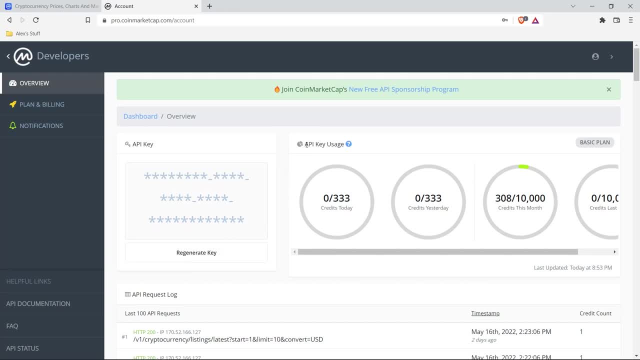 use it for different stuff. or you just need a new key And we have our API key usage. Now you cannot just call it all the time forever. You have limitations, And this is pretty standard with most APIs. They don't want you just overloading their system. right, You're going to have credits, So we 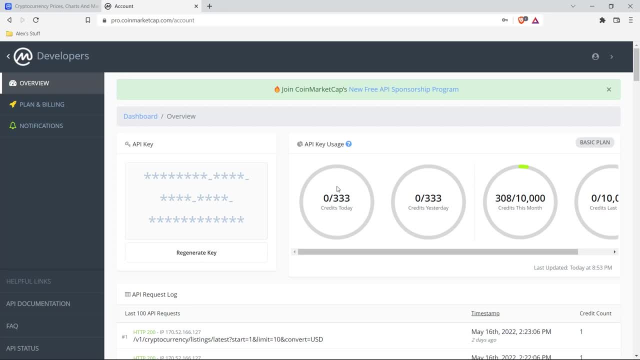 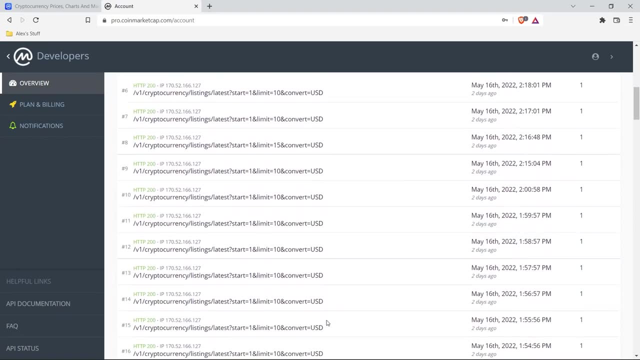 can only use this 333 times today, which is really generous, And so you know we can use this and call this a lot of different times. As you can see, I've called this many times. I've tested this quite a bit. 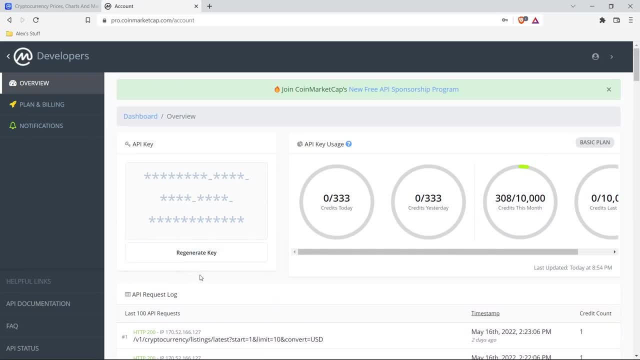 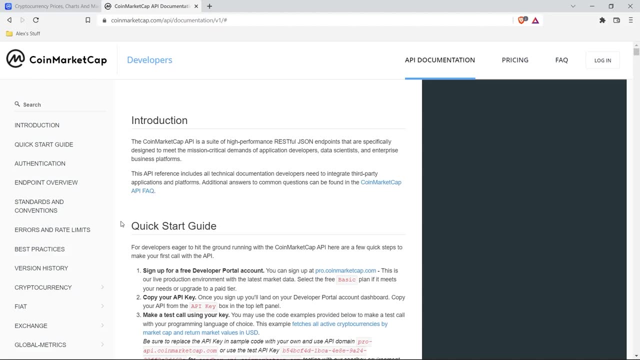 And this is fantastic. So we're going to come back and use this key in a little bit. One thing that you should always look for when you're using an API is the API documentation, which is right over here Now. the documentation for an API can be extremely important, because not all APIs are. 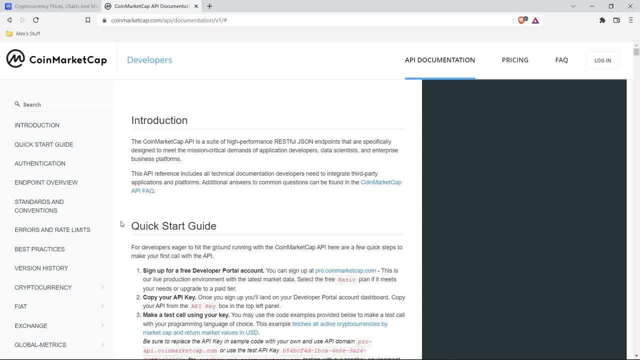 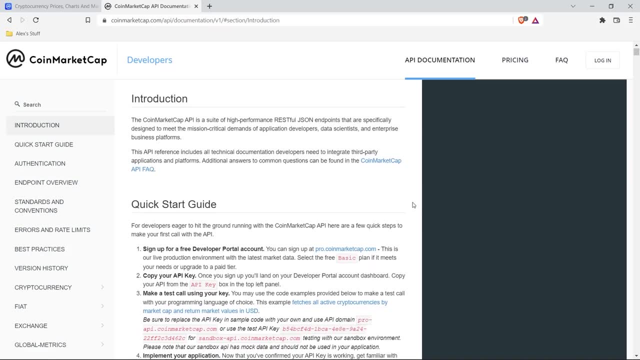 set up exactly the same, And so they're going to show you how to access it, how to use the keys, And it's really important that you read through this, because they may have certain limitations or stipulations on how to use it. So, for us, we're going to be using this and we're going to go to. 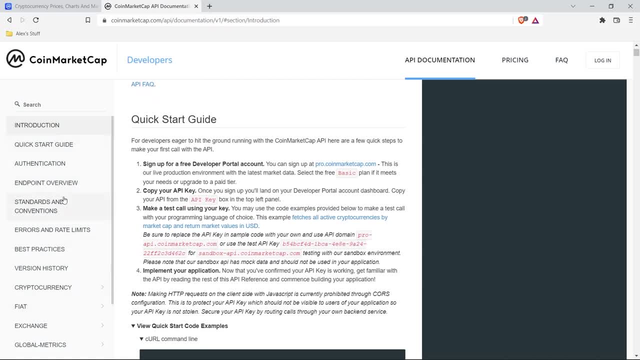 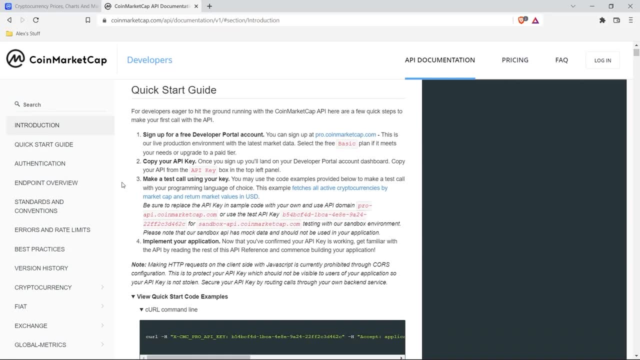 this quick start guide And I do recommend going through all of this. I did, But for the purpose of this video we're just going to take a really, you know, high level glance at this. So right here, we're going to go over here to Python. This is under the the quick start guide. 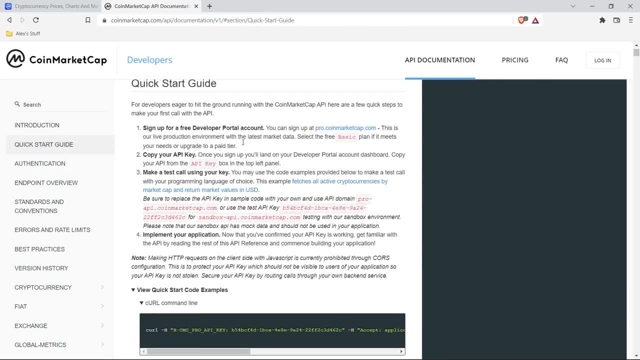 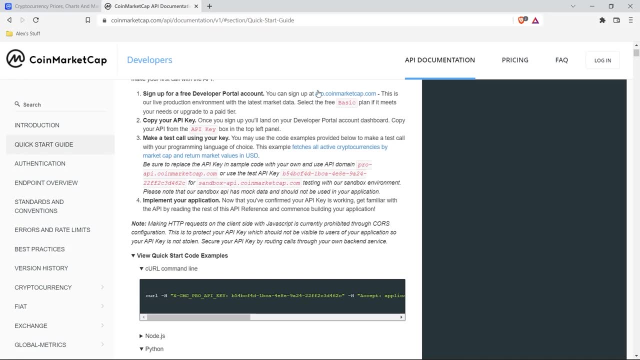 right here, So they're going to show you. you just need to sign up for the free account, get your API key, make a test call using your key and then you can switch it over to the the pro coin market cap later, once you actually want to head off the production environment. 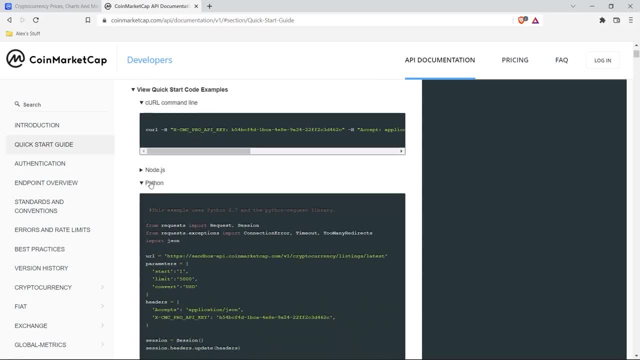 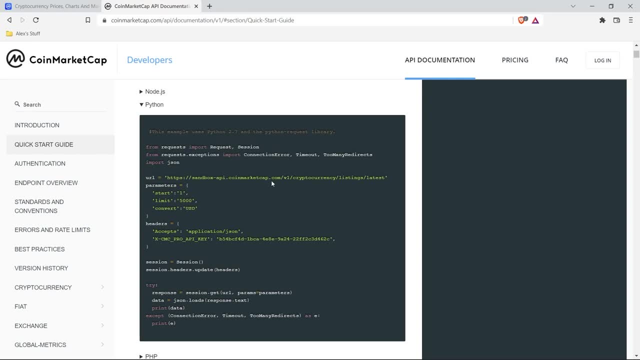 But they want you to kind of test it out first. So I clicked on this Python and they are extremely generous in that they provide you with this code right here that you can just copy and paste and use right away, And it uses this Sandbox API to make sure that your your actual key right here is working properly. 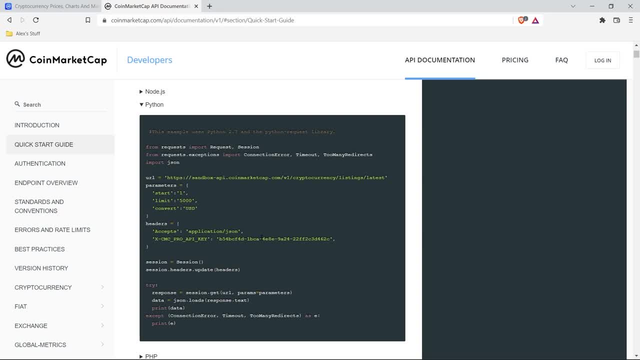 So what I'm going to do really quickly is I'm going to pull up a Jupyter Notebooks and we're going to test this and I'm going to show you how to actually use it. All right, so I have my API test notebook right here. I have my API test notebook right here. I'm going to go ahead and 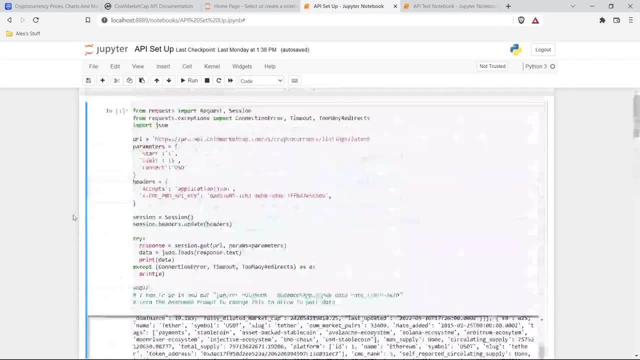 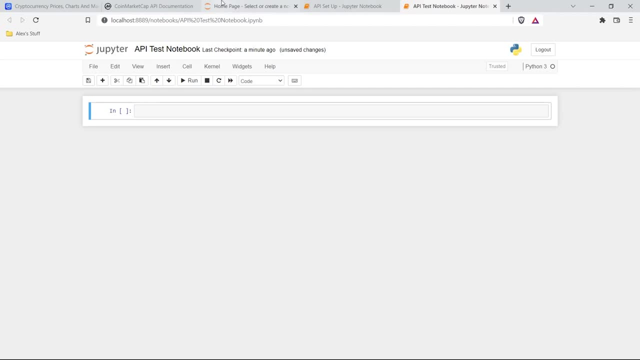 here I have my API setup, which I've already done all of this, So I'm just going to show you how to do it. I've already done all of it, So I might copy and paste some stuff to save me some time, But what we're going to go back and do is we're going to go and copy all of this. Oops. 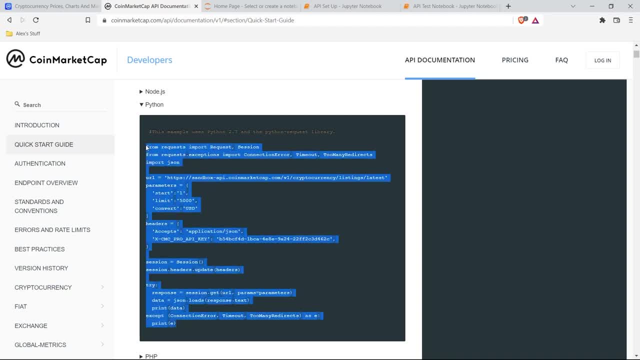 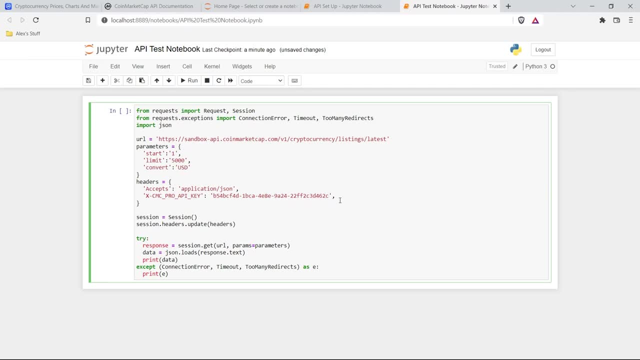 Let's copy this right here And paste it into here. Now, this API key right here. I don't know if it's going to work. Let's test it out really quick. It does work, but that's not our API key. 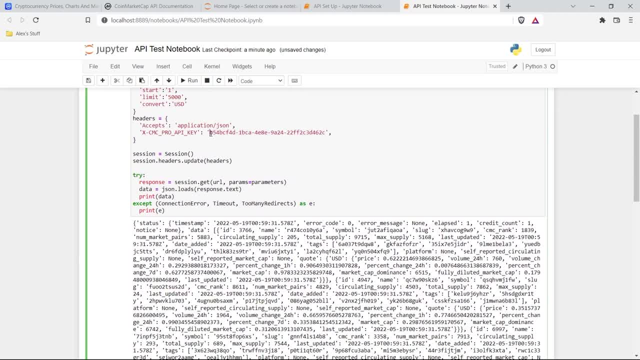 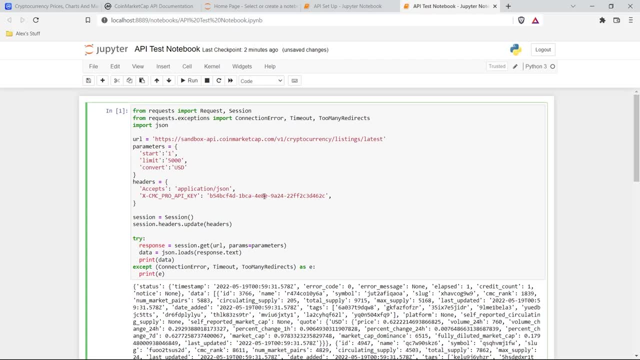 I'm guessing that we can't just use this forever. This is just the one that they want you to use in this sandbox environment, But we want to use our actual API key so that we can make those- you know- 333 calls each day, And then what we're going to do is kind of go a little above and 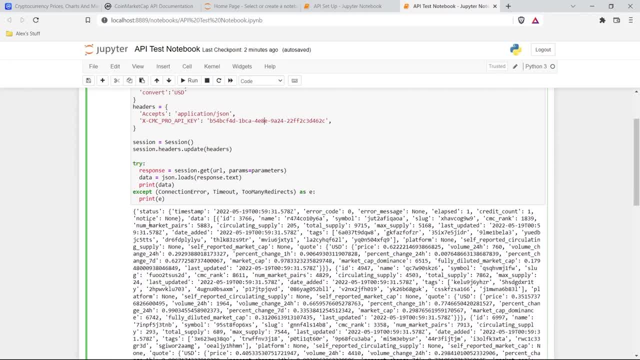 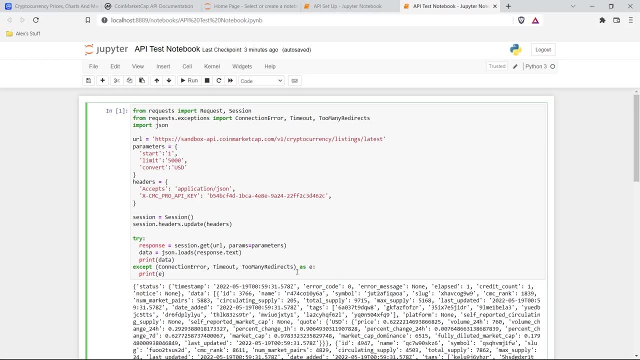 beyond that, to kind of standardize the data, because, as you can see, this is not super usable in its current state. And then, after that, we're going to have all the data ready to go And we're going to set it up for a future video which I create. an entire project around automating this and 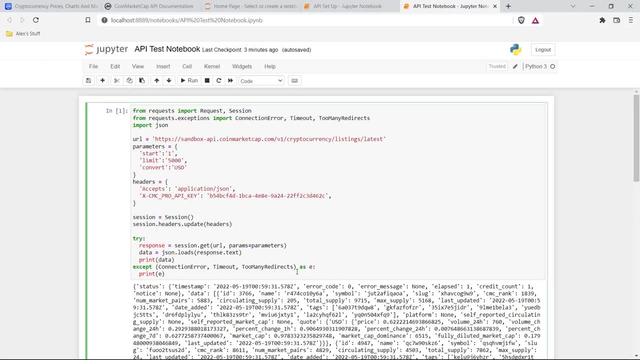 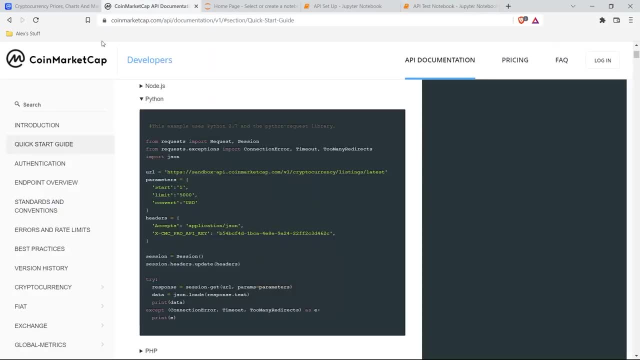 creating automated polls every hour or day, And then we can create the dashboards for it, And it's going to be a fantastic project in my opinion. So let's go right back up here, And we are going to go back so that we can grab our API key. So this is our unique API key. we're going to copy. 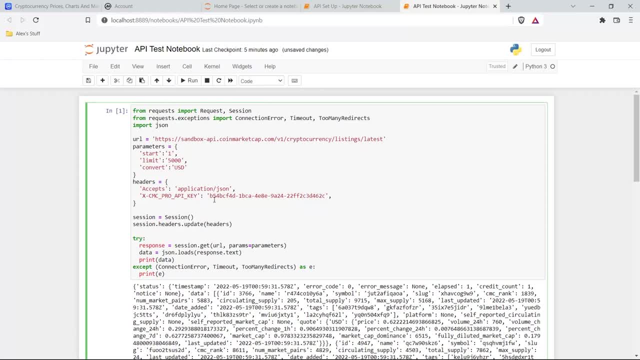 that And we're gonna come right over here And we're going to paste it right where it says pro API key. Now, this is my unique key, but feel free to use it. I created a dummy account So you can use it. I'll provide all the code in the description. you can go and click on it. download, you know. 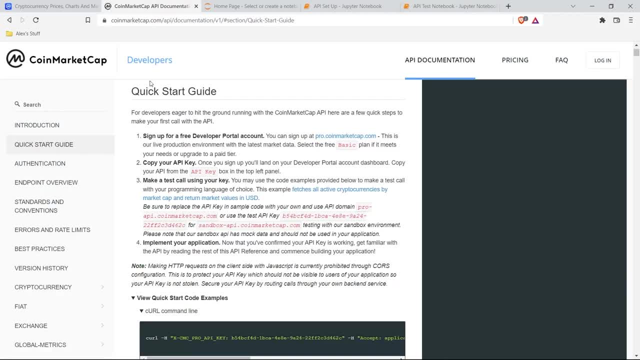 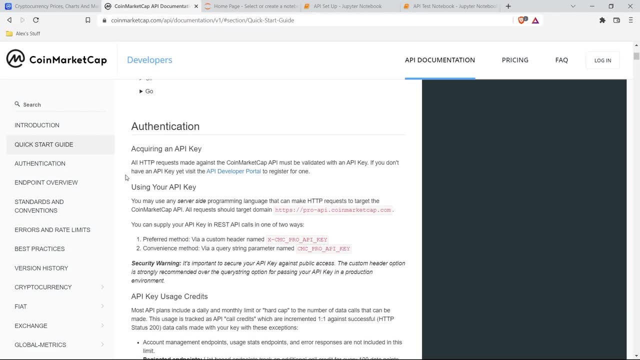 the code and use exactly what I have Now. if we go back to the documentation right here and we scroll down just a little bit, this is using the sandbox API. But if you come down just a little further, it's going to tell us how to actually use our API key And it's going to say: 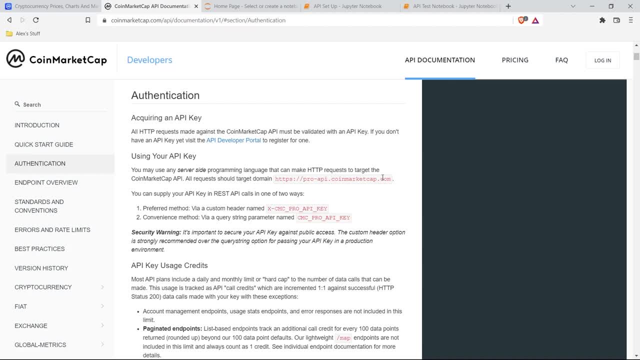 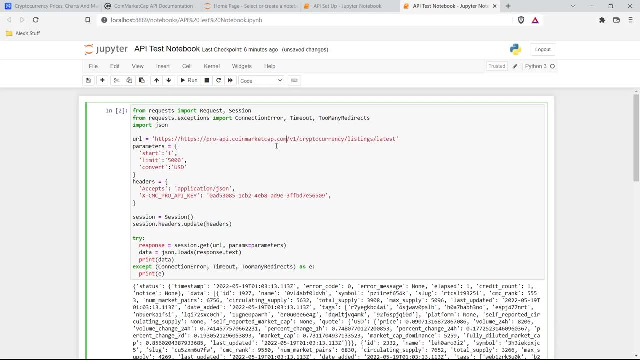 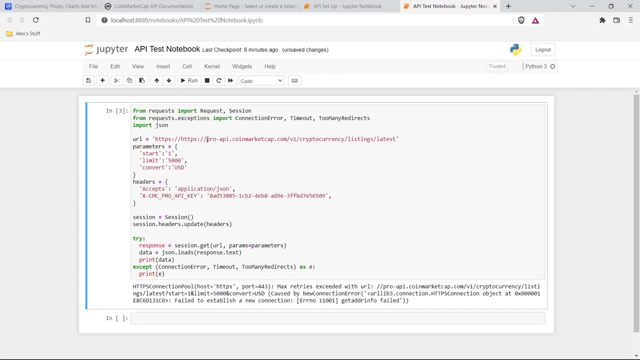 that we should target the domain of pro dash API. So let's copy this And let's go right here And let's see if it works. And it failed- And I think I know the issue- I need to get rid of this right here. So now let's try. excited to, HTTPS is in there, So now let's try this. 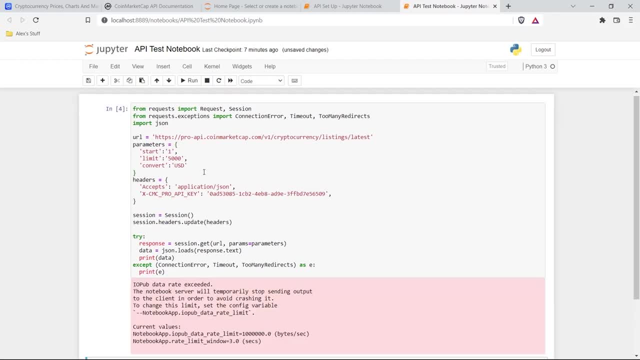 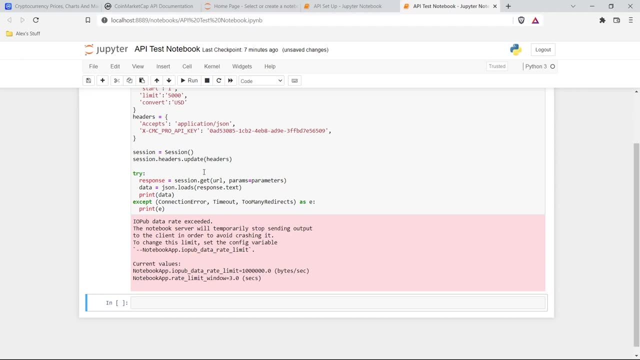 and see if we can get the data using the correct HTTPS. So I was hoping that this was going to happen, because this is exactly what happened to me the first time I tried to pull data from this coin market cap, And I haven't had this happen in a long time, And I wanted to show you. 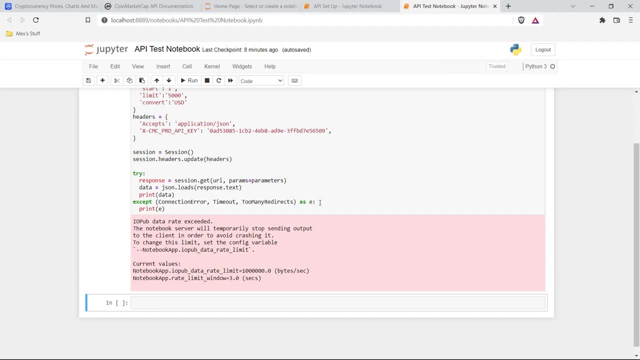 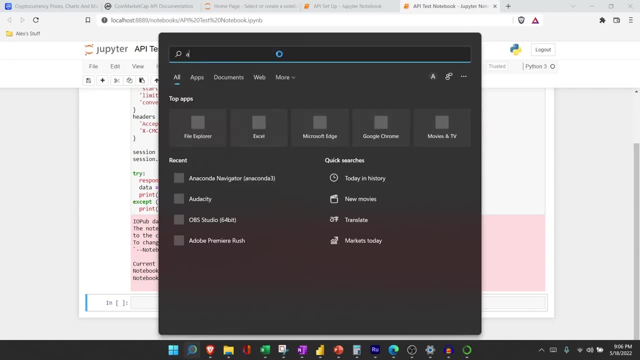 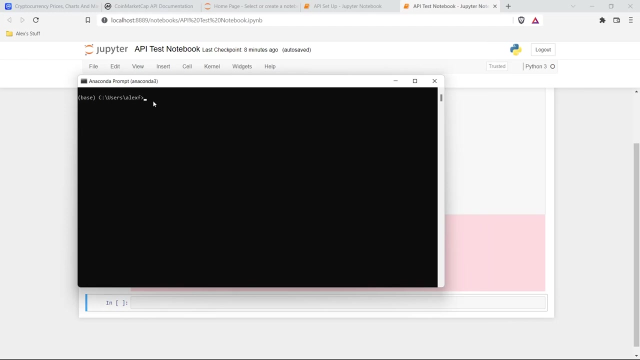 how to fix it. So I'm honestly glad this happened. So what we need to do is actually increase the data rate limit. So what we're going to do for that is we're going to search and we're going to say in a condo prompt: And when we go in here- this is for me at least- we're going to paste. 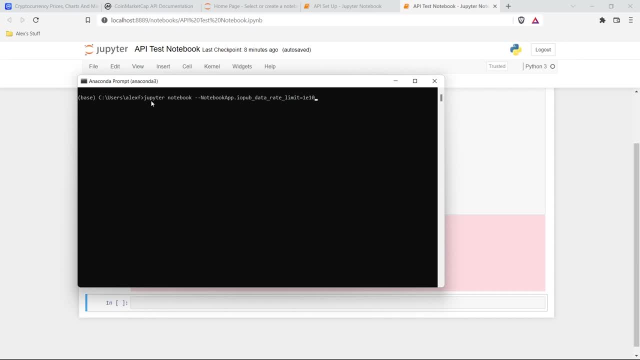 this right here And I'll have again. this will be in the, in the code that I offer you it'll. it'll have this at the bottom you need to put in Jupyter Notebook And we're going to increase the limit of the data that we can put in here And we're going to paste this right here And 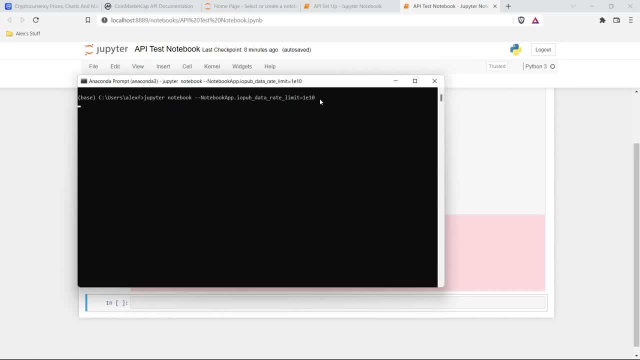 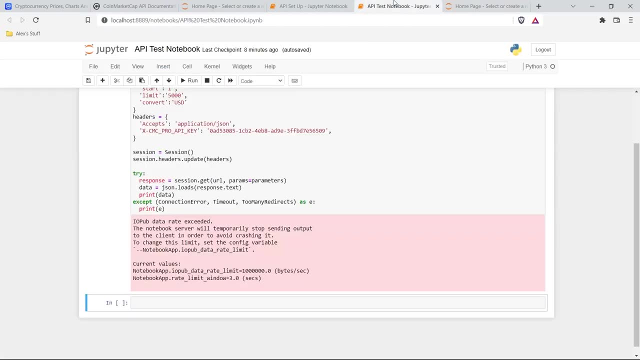 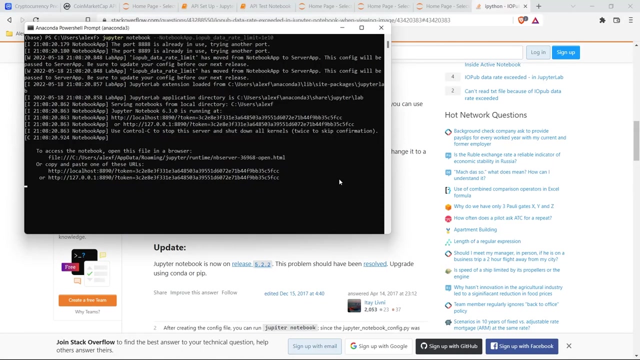 we're going to hit enter And it's gonna do a bunch of stuff here. Give it one second And I think it fixed it. Let's run it and see if it worked. Alright, so this obviously didn't work like it did last time for me, which would did not see coming, if I'm being honest. So I am on. 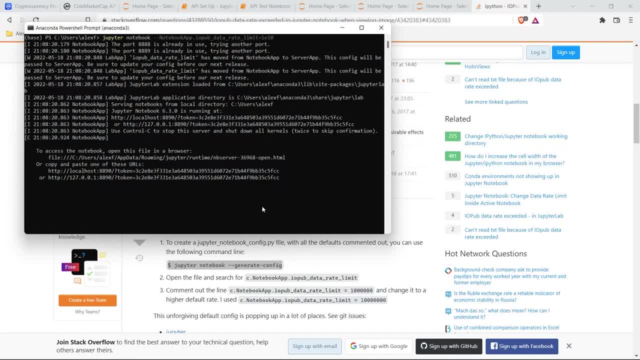 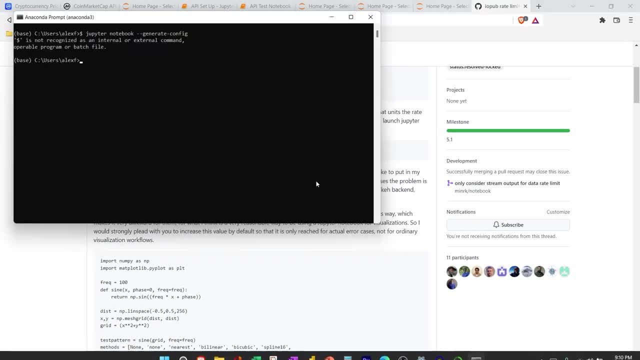 Stack Overflow trying to figure this out. I'm going to kind of walk through this with you and see if we can figure this out together, Because if this happens to you, it'd be really great if you know this would help you figure this out. Alright, now I have this other. 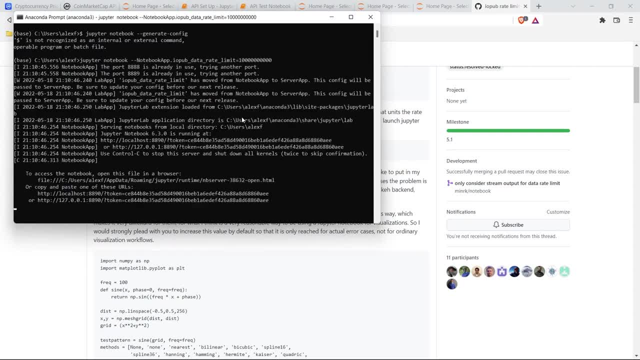 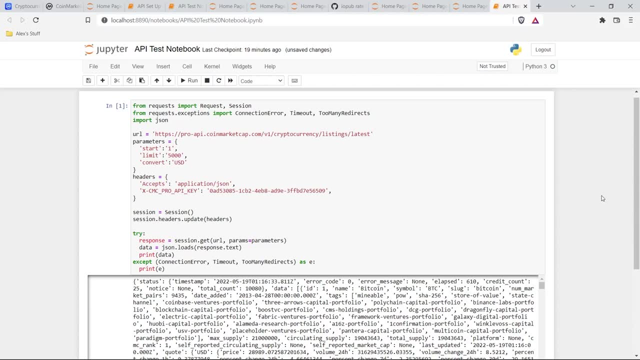 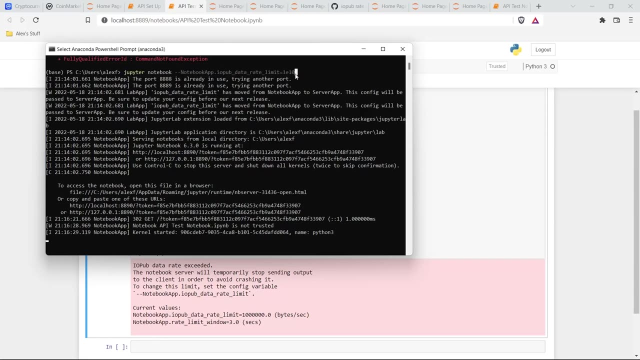 one telling me to put this in, Let's see if this one works. No, that didn't work either. Alright guys. so I got it to work. I it was honestly by dumb luck. If I'm being completely honest, what I would do is try using this right here. That's what I did And it worked. 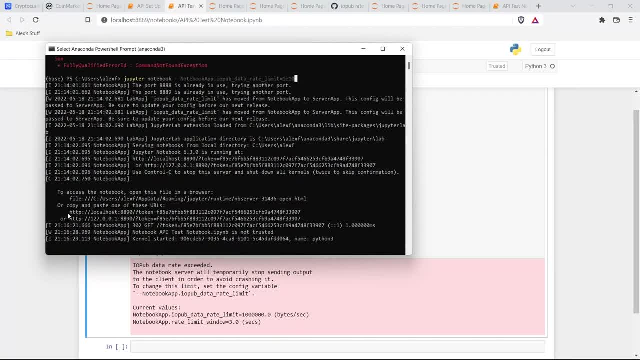 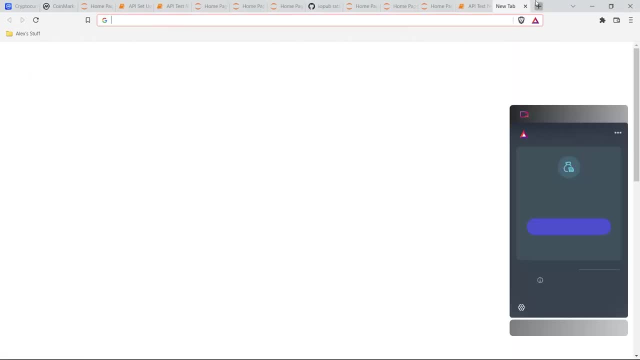 But what I ended up doing is I just copied this localhost. I said copy or paste one of these into the localhost, So I was like, Hey, let me try. So I copied it, I put it up here, I went over here. 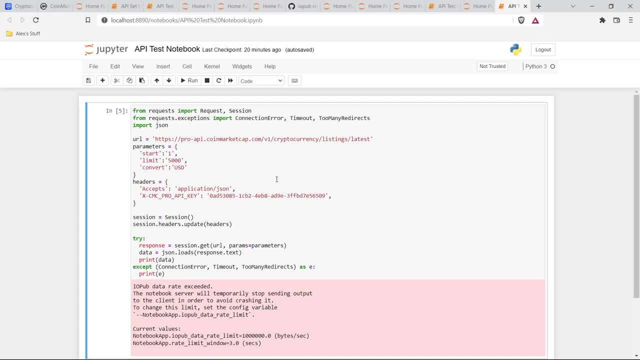 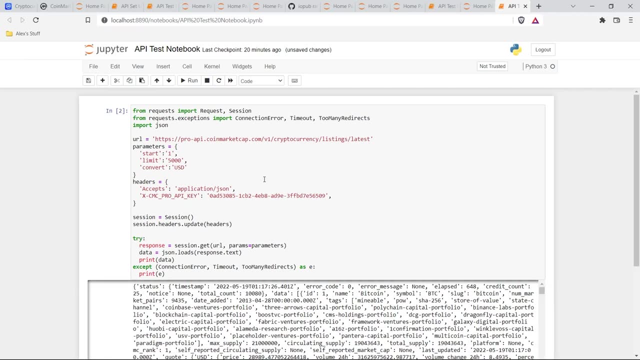 to API test notebook, which is the one that we're using, And then I ran it again And it worked Again. the half of this stuff is just like tinkering with it and figuring it out. If you've ever watched one of my projects, I show that stuff because this stuff is going to happen And so just 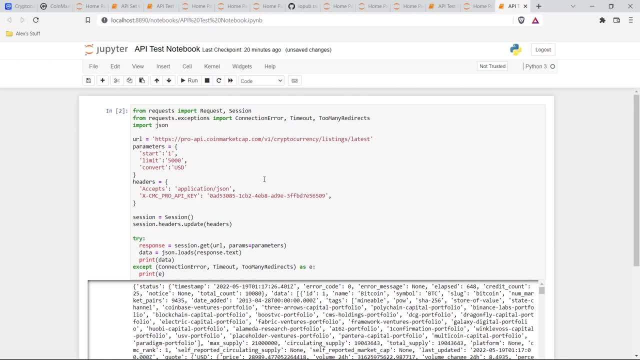 a warning that if you're trying this and if you're actually using this around the code, you may encounter that, And those are the steps that I took to figure it out. As you can see, I have a ton of stuff up here from all my testing over the last like 30 minutes. 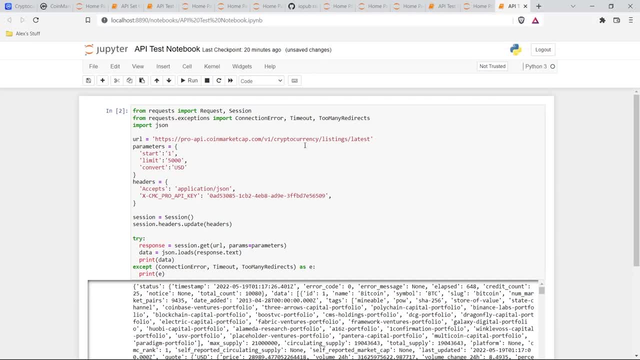 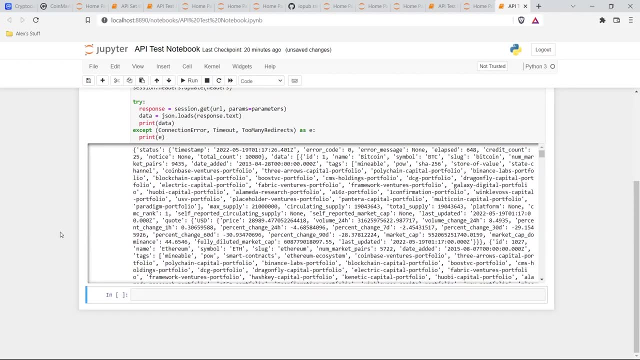 try to get this to work, But now it works. So now that we have the actual data in here really quickly, I'm just going to show you how to normalize it and make it look a little better. So, if you can see, this is actually in. 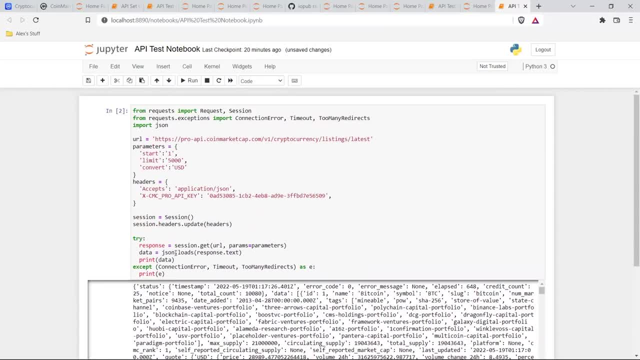 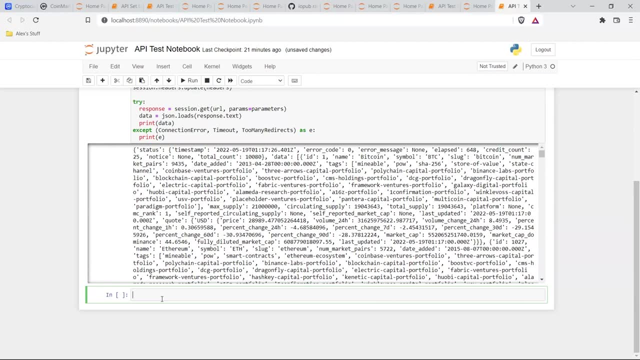 this JSON format. So use this JSON dot loads And in order to get it kind of into usable state. but you know we're I'm going to show you how to do that, But just to show you. this is a type and we're going to the. this is data, right here. 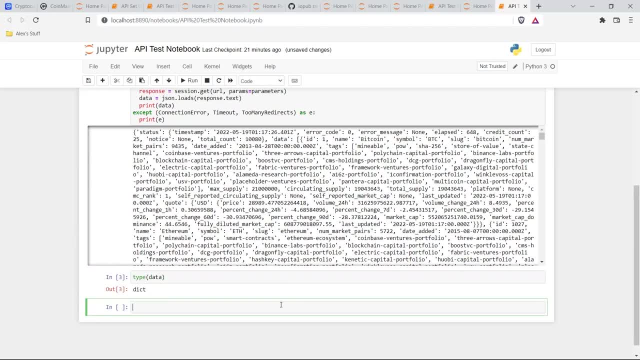 Type of data. it's in a dictionary format, data type, And so we're going to do is import pandas as PD, And then we're going to do PD dot set. Well, let me show you this in a little bit. Actually, I'll write a. 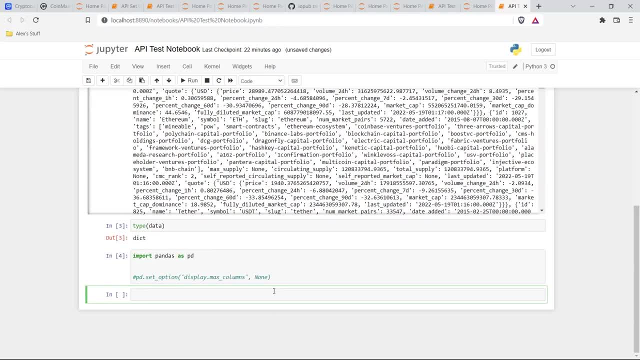 Now that we have this, we're going to import pandas, And what we're going to do is we're going to do something called a JSON normalize, which is just going to make this look a lot prettier- And you'll see that in a little bit- because basically going to put it into a data. 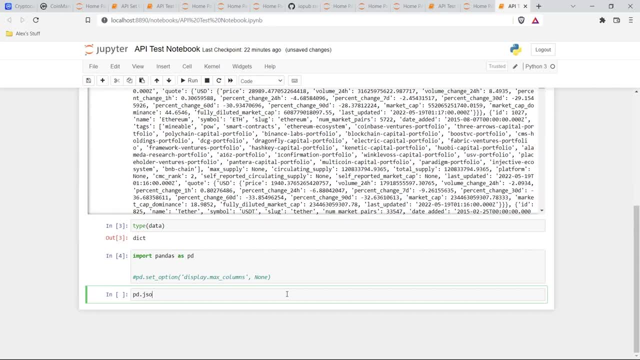 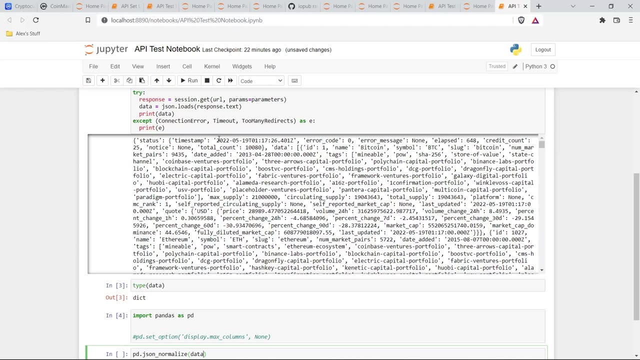 frame. So we're going to say PD, dot, JSON, underscore, normalize, And we're going to say data, And I know I haven't really showed you this data super well or everything in it, But in the inside this, this JSON, which is kind of like nested, there is data in here. let me see if I can. 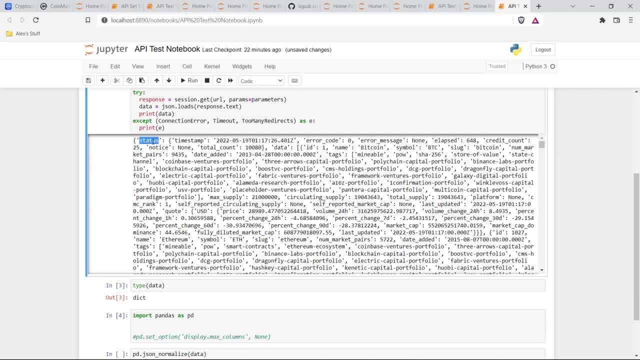 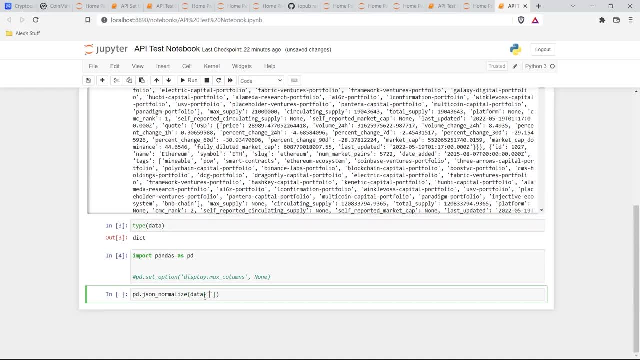 find it. So we have the status, so we can pull in the status, which, for the sake of it, I'm going to show you how to do that And you can see some of the data that we can pull in its status. Let's: 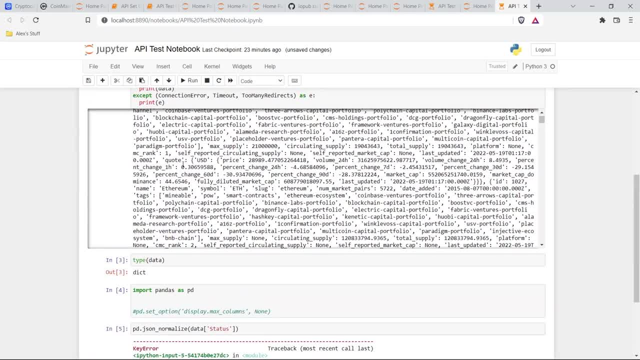 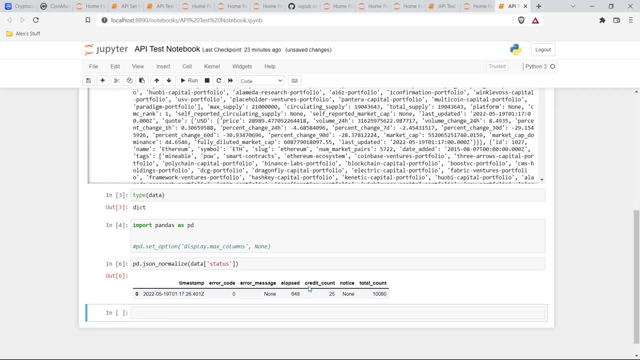 try that real quick. I think it was capitalized. Oh, it wasn't. Let's do that. And this is the data that's pulling in. This is a timestamp, this is the error message, the total count, some of the things that you see right up here. right Then, right here we have our data. Now, this is the 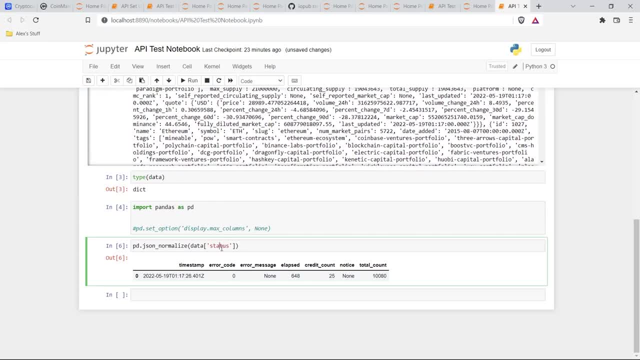 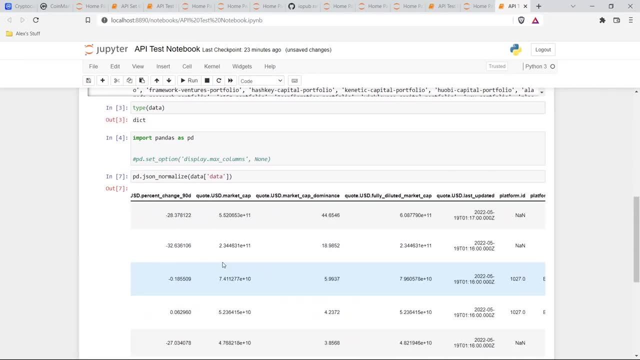 actual data that we want. So let's pull that in And, as you can see, it is much, much better looking than it was just a second ago. has all the things that we want. As we can see, we have Bitcoin, Ethereum, Tether, oops, And so we have all of these things Over here. we have 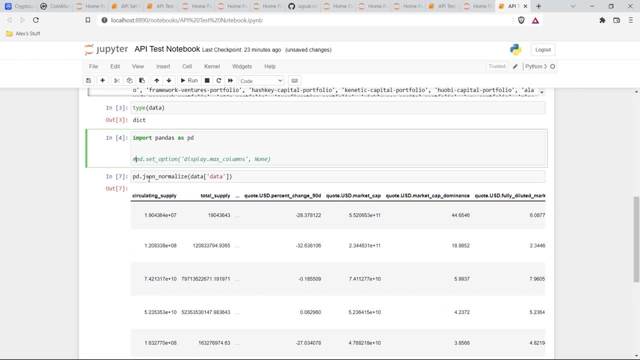 this, dot, dot dot. That's what this right here is. So what I'm going to do is I'm going to run this again And now we'll run this again, And now we should be able to see every single column. 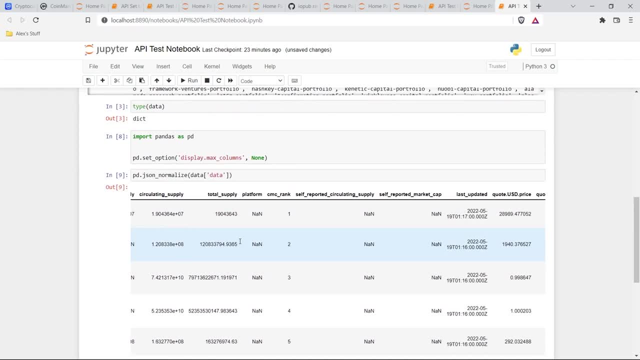 That's what this does: It displays the max columns. So now we can see every column And we can look at the last updated. This is today's date at today's time And here's the price, So we now can look at. 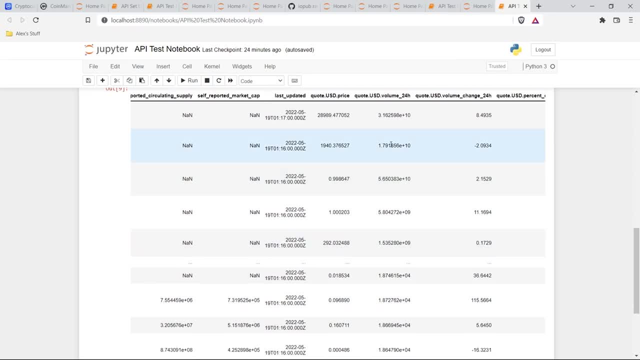 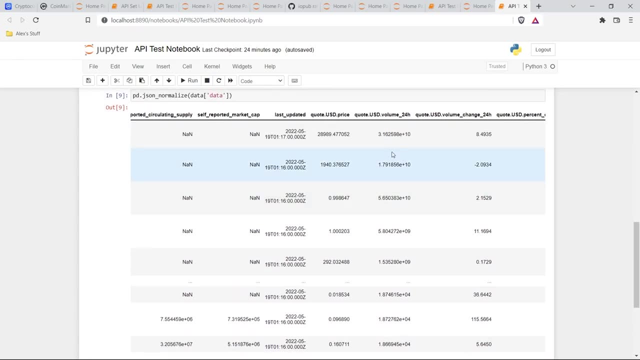 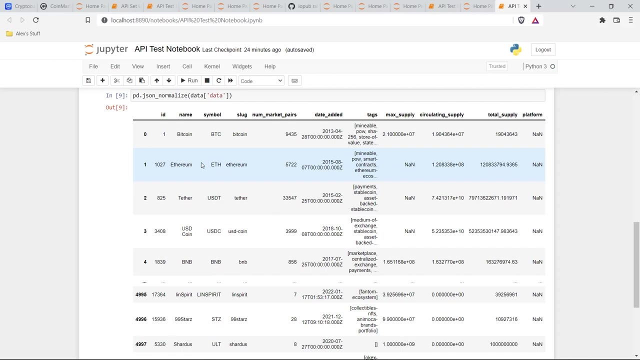 the price. You may be seeing a lot of standard notation on this and you may want to know how. I'll show how to do that in the future video when I make the full project out of it. But that is how you use an API. Now we have all this data. We can put that into a CSV. We can keep it in the data. 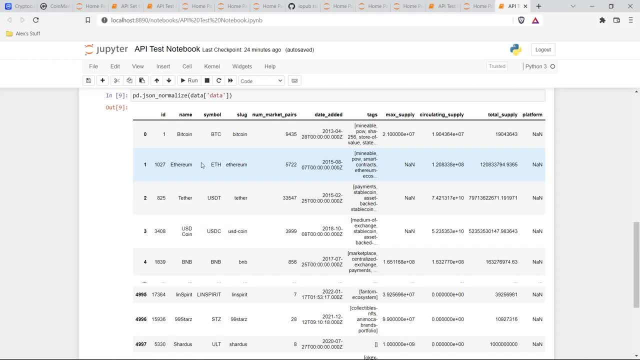 frame. You can do whatever you want with it. You can then use this and put this into a website so that you can display this information on your website. There's a lot of things that you can now do with this data, And that's how you are able to kind of connect to this And you're able to use. 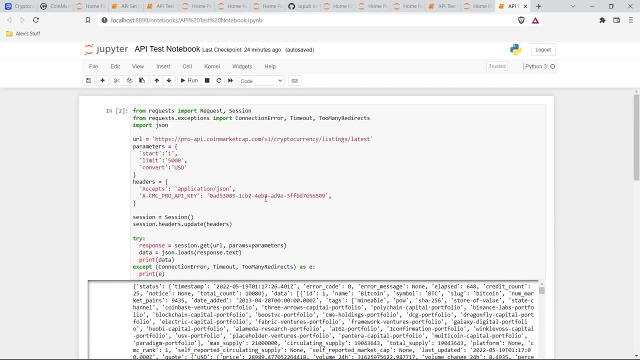 this key to access their API. Now again, I didn't have to do almost any of this or write any of this, because they already had it all written for me in the documentation. So I highly suggest reading a lot more of that documentation.